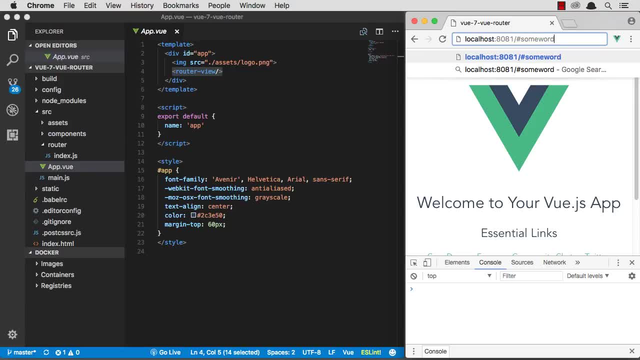 hash and then some word. here HTML will look like this. It's going to look like this: It's going to look for an ID on the page called some word and it will scroll to it So you can actually make a URL. Any link on the page could link to hashtag some word and that would actually scroll to the 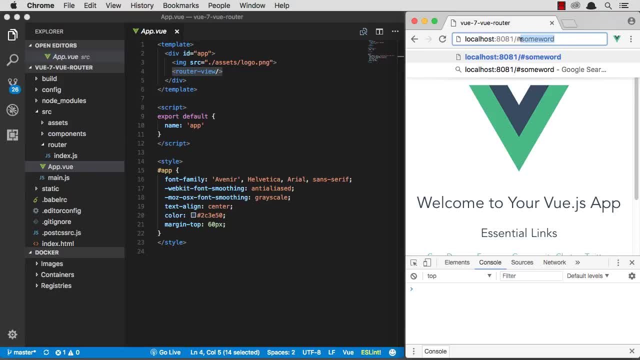 some word ID when you click on it. But then developers learned along the way: hey, since it doesn't navigate to a different page, we can kind of hack HTML and add all this information here, And then we can listen for when that changes and tell a JavaScript application to go to entirely. 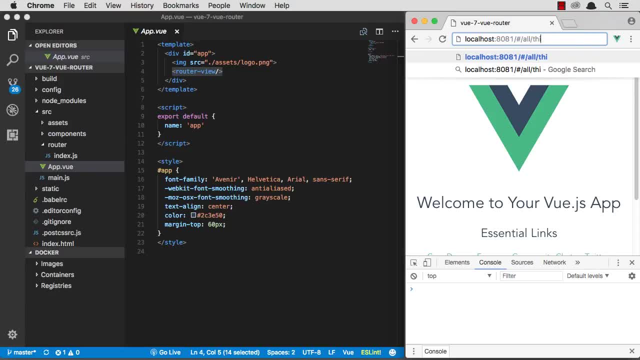 different pages, States and stuff. So that's basically what the concept of routing is is we're going to add information up to that hashtag route, And there's an HTML5 way to do it too, but we won't cover that in this video. But as we add stuff to that route, JavaScript can pick up on that and we can make the 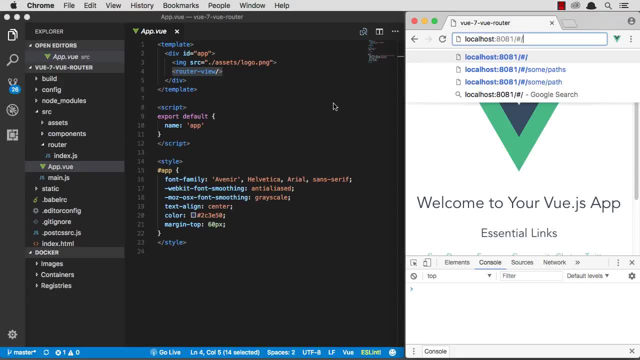 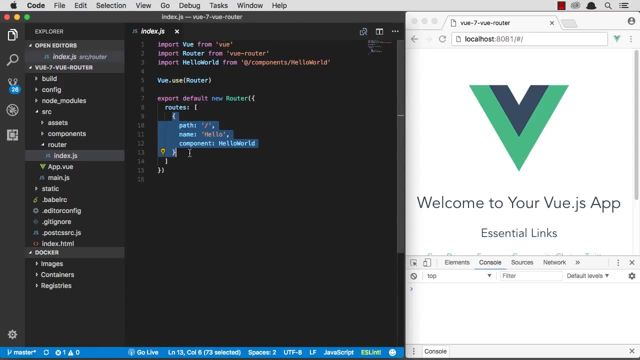 whole page change without navigating away. So there you go. That's routing for beginners. So here's what that router view covers is: we can define a set of routes And when you go to those routes it will actually load a different set of components. 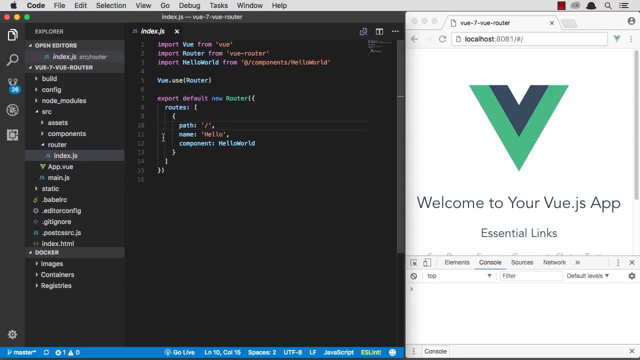 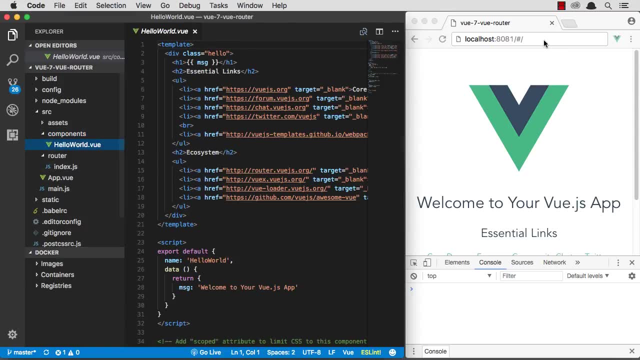 So you can see here, when you're on the slash route, just the homepage route, we're giving it a name. We're saying, hey, that's the hello world component, So that's the hello world component right there. So if you go to just slash, it grabs the hello world component and it spits it out in place of 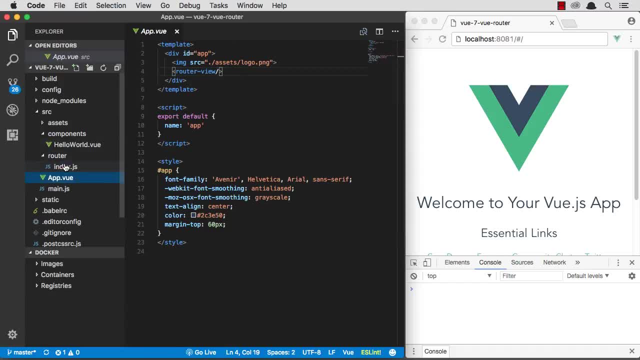 router view. So that's kind of how routing works. Let's go ahead, define maybe another route here Let's say, oh well, let's, let's show you one thing here. So if I go to a fake, fake path, 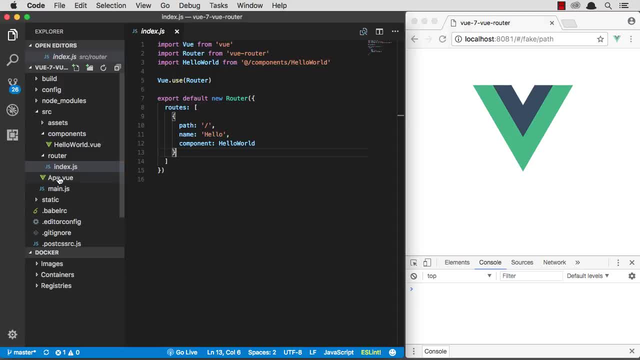 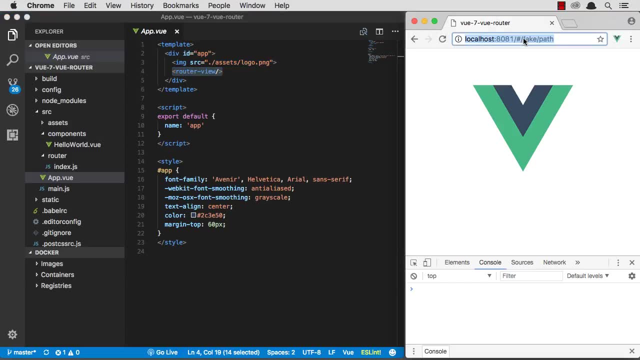 then all you're getting is the top level application. at this point You're getting app view, which is the div and the image, And this is returning nothing because there is no router view for this, So it's basically returning no component at all. 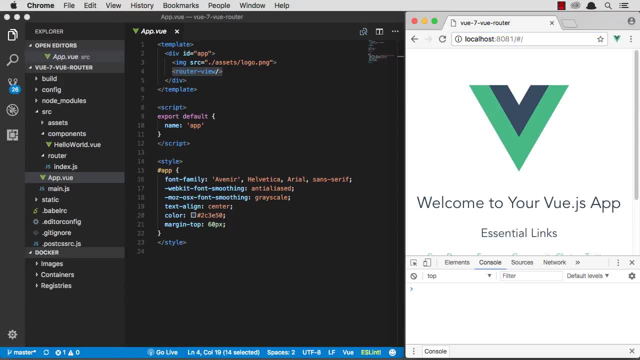 And then, anytime you go to something that the router view recognizes, it's going to return that component, which case? this is the hello world. So you use the app level view for a shell for your application. Whatever is going to apply to your entire application goes in here. 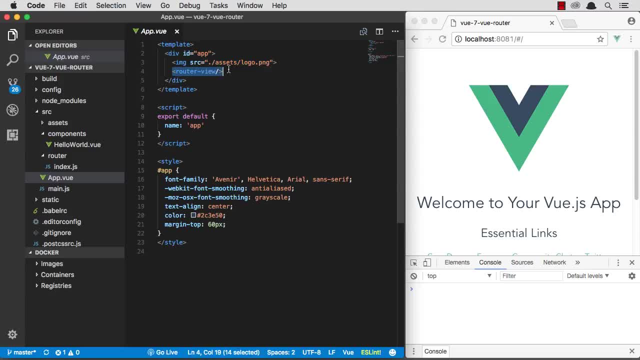 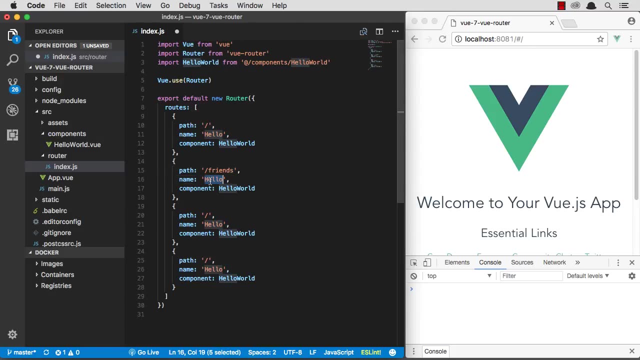 every single view state And from there you break down different things into views. that router view can then return. So let's go add maybe a. you know. let's say, we were making that friends list. Let's do a contact, We'll go friends. So that's our friends path. And then 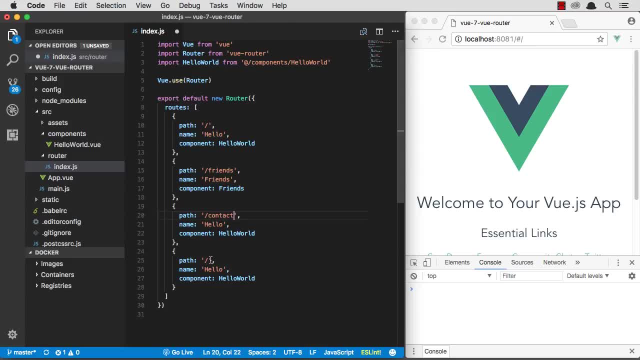 we could also make, say, a contact path, And then maybe we can make an account path where you can manage your account or something like that: Contact accounts. This would be the contact components And this will be the account components, And you can get more complex than. 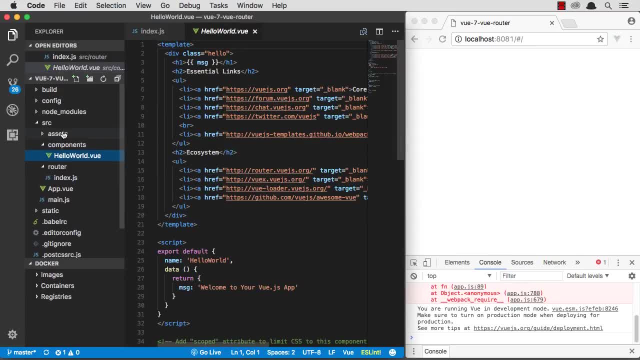 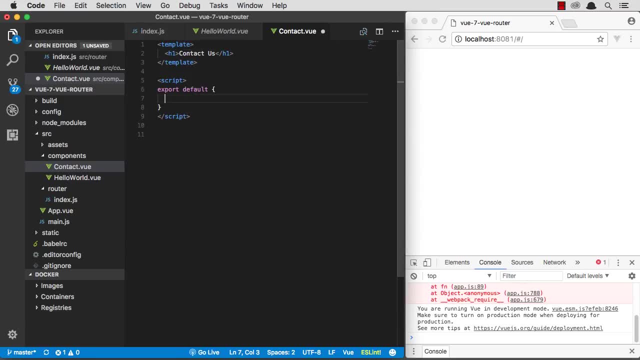 this. There we are. Let's go ahead now. Just make some new components here. Contact view: Let's go ahead and make this And we'll just leave that as that. Let's go ahead and save this also as the accounts And let's save this as friends. So change a couple H1s here. 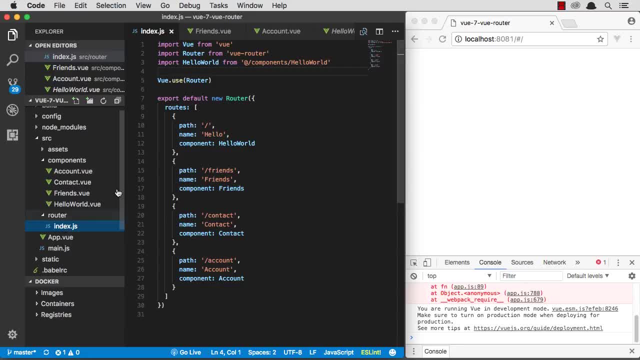 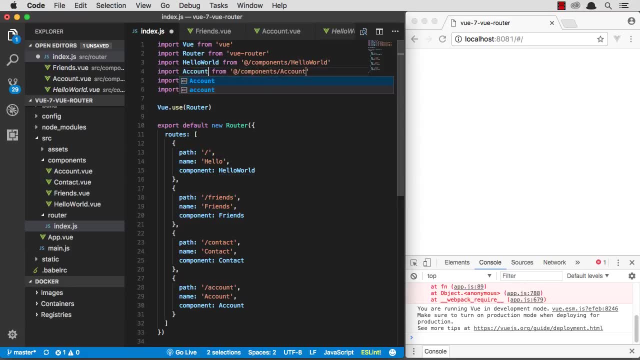 So now, if we go back to that router file, we can import those files we just made, We can import accounts, We can import contacts And we can import friends. Everything should be working now. So now, if we go to accounts, we get the account component. 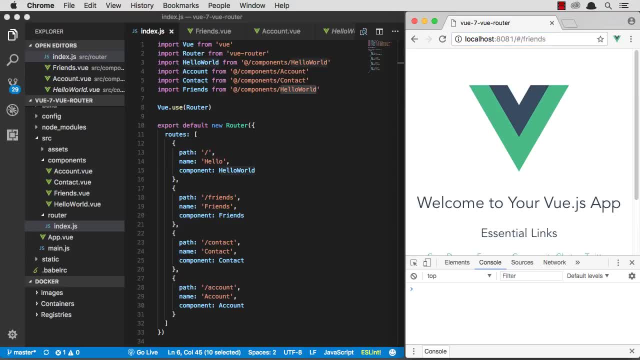 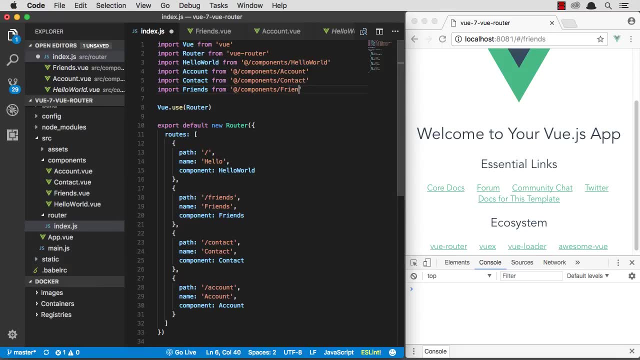 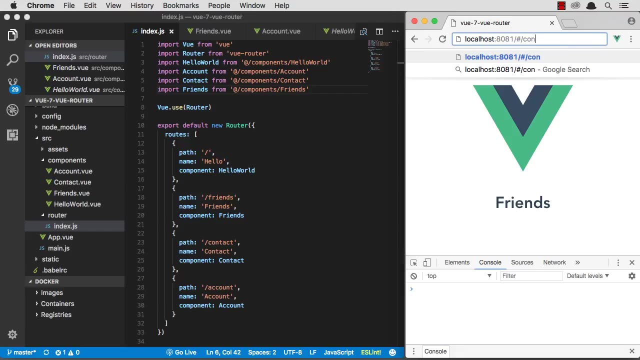 There's our account H1.. And we can go to friends. Whoops Looks like friends is the wrong component. Yes, we are importing friends from Hello World. Let's change that. There you go Now. hash friends, Hash slash friends goes to the friends component And contacts. So there we go. That's all of our. 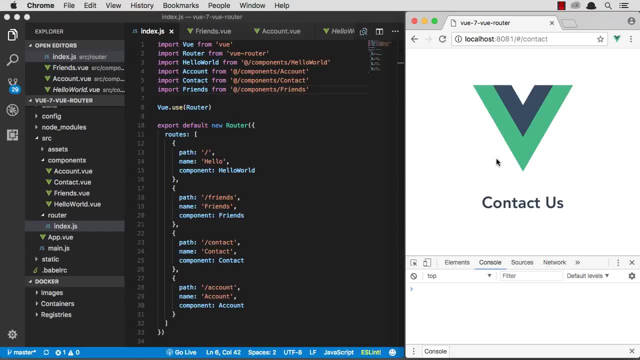 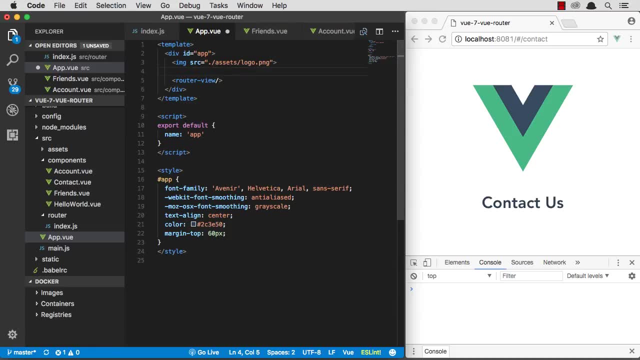 pages. Now let's go ahead and create some links here So we can actually link around to these different pages. If I go over to my app view now, I can go ahead and create some links by using the router link tag- Router link- And this is basically an A tag, So I can go to the front page And I can 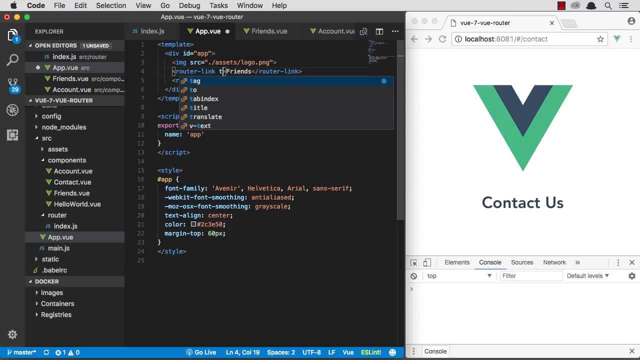 go to the friends And all I have to do is add a to And then I can basically give it the path I want to go to. I can go to friends And let's also do accounts And contacts, And I'm assigning these to. 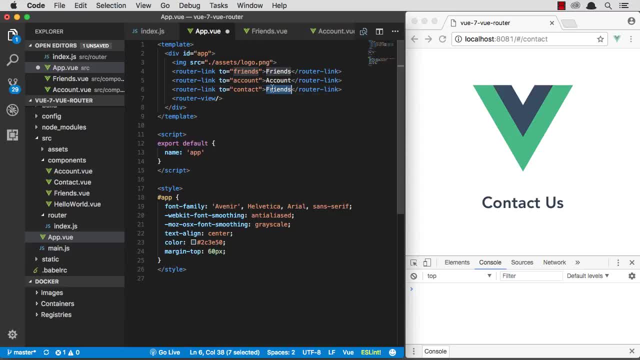 the top level application. So that way every view I go to will have this main level navigation. So now I can go to friends accounts or contact. Excellent, That works well. I can also add extra details in here, So I could go friends- slash one, slash two. 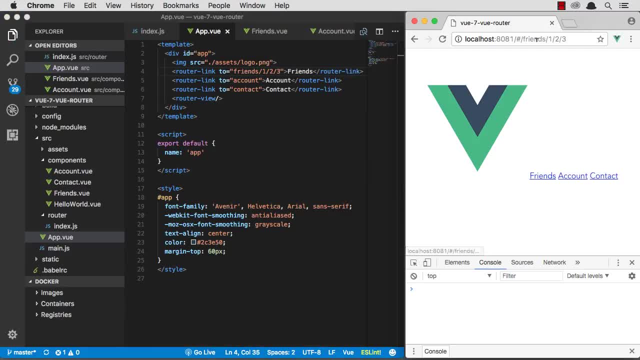 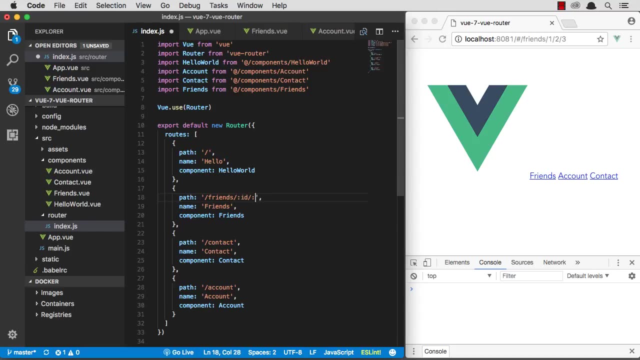 slash three. Let's go ahead and save that. So if I go to friends now, you can see it goes: friends slash one, slash two, slash three. But there is no route that matches that. What I can do is I can come over to my router index And I can go: friends slash ID age. I don't know weight, Let's say the. 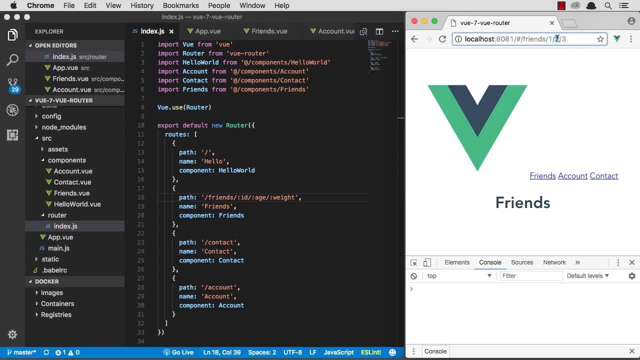 weight is particularly important. So now this would be the ID And I can go to friends, slash ID, the age and the weight. That makes absolutely no sense that you would load a friend by ID and pass in an age and a weight. But whatever, At any rate we are passing this in And then we can then 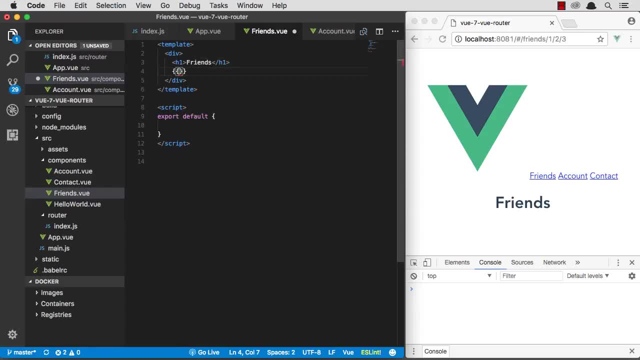 access those in the friends view. We can come in here And we can do routeparamsid And you can see there's ID. one gets spit out And we can also access route params- age and weight. That is it. This is a very light two-year-old And there's another way you can do it If you want to validate. 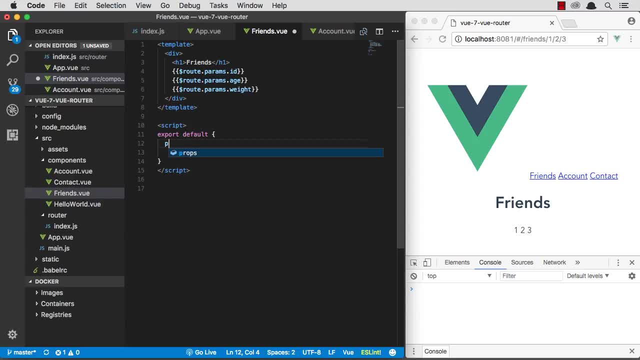 that by adding props in here, then I can actually require those this way. instead, I can add ID, age and weight, And you can also add validation to those, So you can require those to be certain types, which is pretty cool, And then I can come over here to my routes And all I have to do is 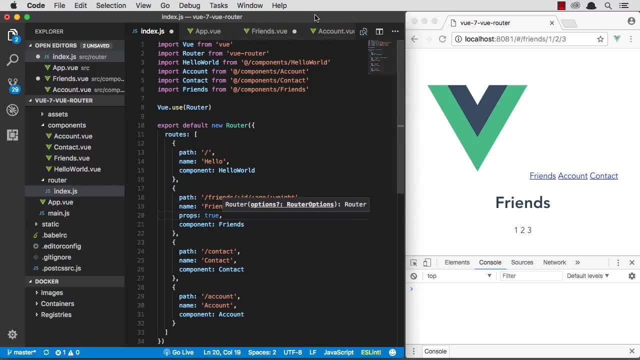 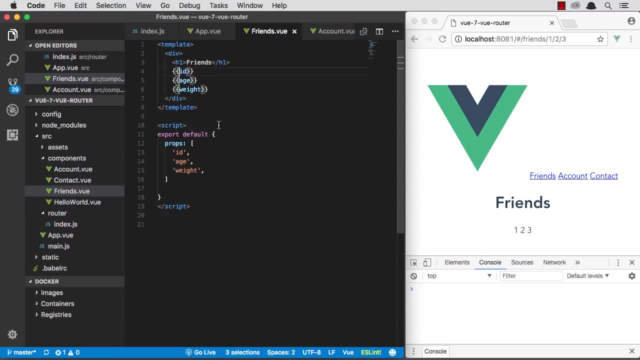 say props, true, And now those get passed in As props. So those will get passed in as props, And now I can just call these age, weight and ID. You see, this will render out exactly the same. Let's refresh, Yep. So now, if I go to a weight of, 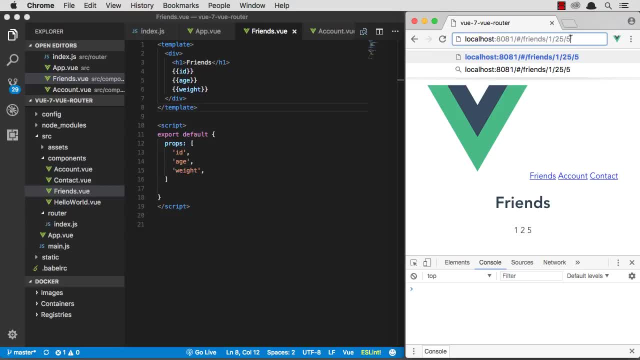 five, age of 25, maybe a weight of 150, something slightly more realistic. all that information comes in from the route and gets passed automatically to the component. So those are the two ways that you can pull in those props And using Vue Router you can.